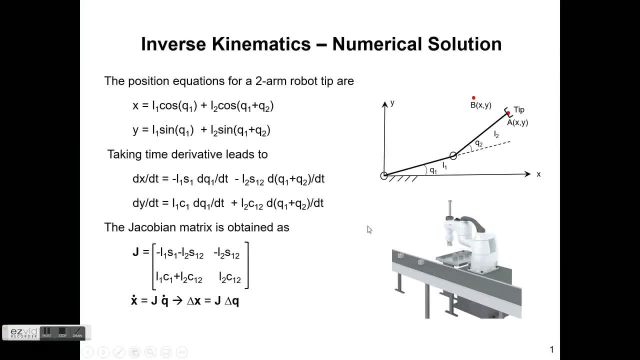 Okay, today I'm going to show you how to do the dissemination for point-to-point control, like for the pick-the-place application, using a two-arm robot. and here is a two-arm robot model, so L1 for joint Q1, L2 for joint Q2 and for given tip position XY and you can. 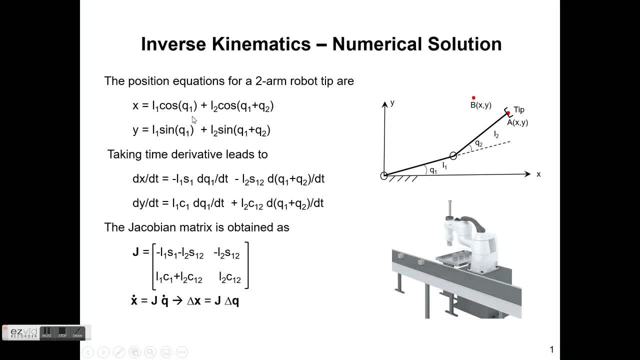 express x in terms of angle L1 cosine Q1 plus L2 cosine Q1 plus Q2, y equal to L1 sine Q1 plus L2 sine Q1 plus Q2, and then you can take a derivative on this equation. so there's a dot x- d2. so sorry, dx, dt, so it's a dot x. 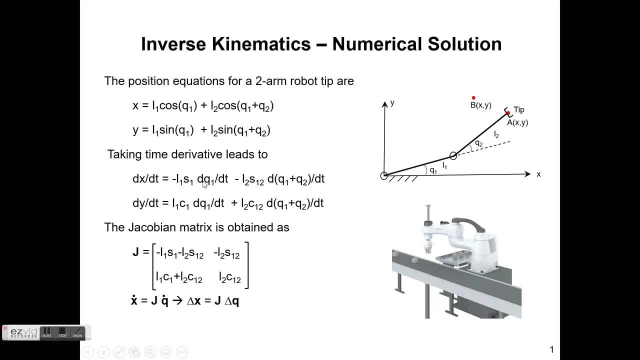 equal to minus L1, sine 1 and dq dt, so x1 is actually sine Q1, which is for short form. and then do this derivative equal to minus L2, sine Q1 and Q2. this is a short form of that. and then that's the dot Q1 and the dot Q2, and then for the derivative on: 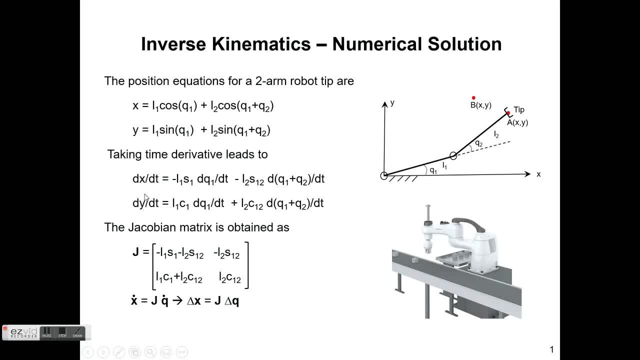 then you have d, y, d, t, and then derivative on sine would be equal to cosine, so L1, cosine, Q1- okay, the short form for cosine Q1, and then that would be a dot Q1. and now here this term would be equal to L2 and sine would be cosine. so Q1 plus Q2 and that would be dot Q1 and Q2. 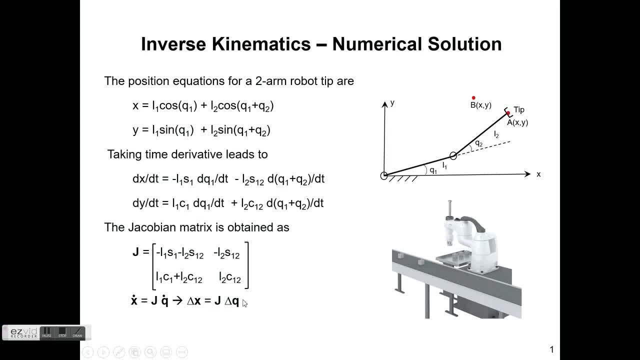 so then from there you can extract what they call the Jacobian. so the term associated with a dot Q1 will be here and the term associated with only dot Q2 will be this term here, and for y dot and the term associated with a dot Q1 will be this term. 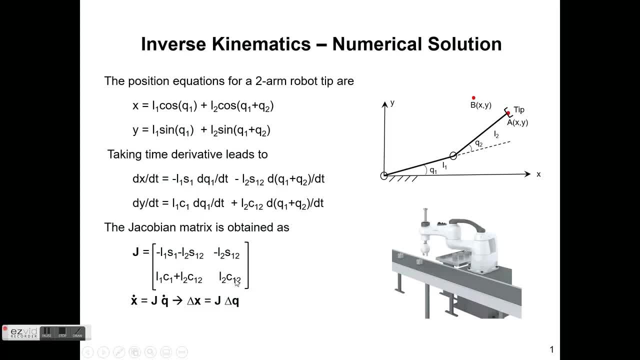 and this term here and the other term will be this term, it will be associated with a dot Q2. so if you use Jacobian and then the uh, the x dot in this case is the vector. so in other words it is a dot x and y is in the vector form is equal to j time the dot Q1 and Q2, so that's the vector. 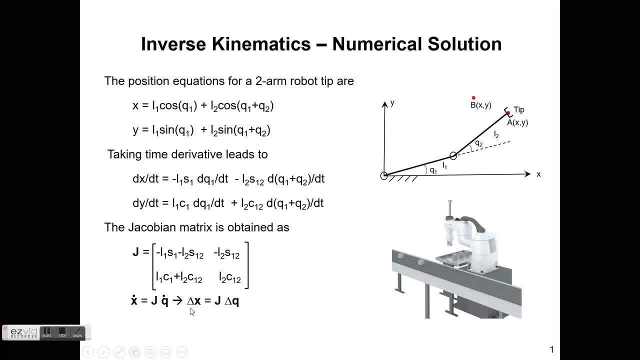 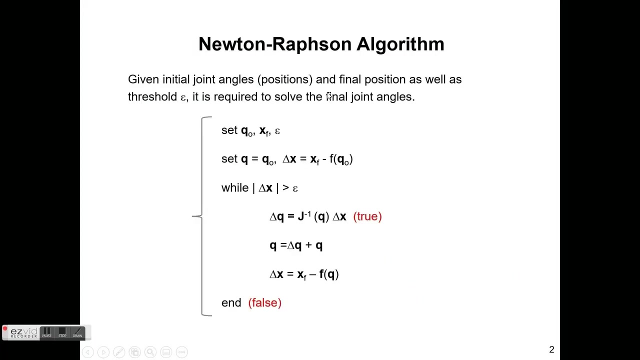 and then if you write in uh, infinitesimal way, so it, because this is dt right, d t cancel, d t equal to delta x and delta q. so, Jacobi, also relate the increment motion of the tip, relate to the increment motion of the joint. so with that we can solve this point on control. 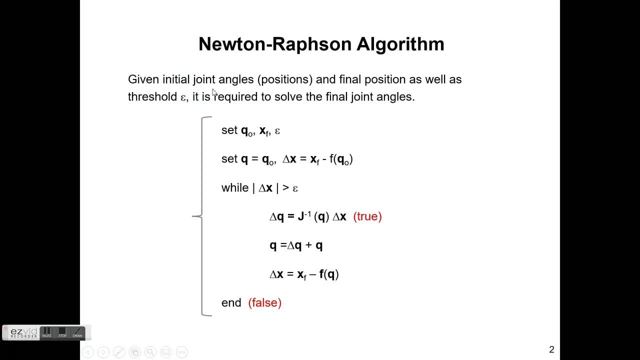 using what they call the Newton-Raphson method. so probably stay like this: if you're given the initial joint angle or position in a final position, as well as the threshold, the absolute is required to solve the final angle, not find which one angle. so this is the quadro quotes. 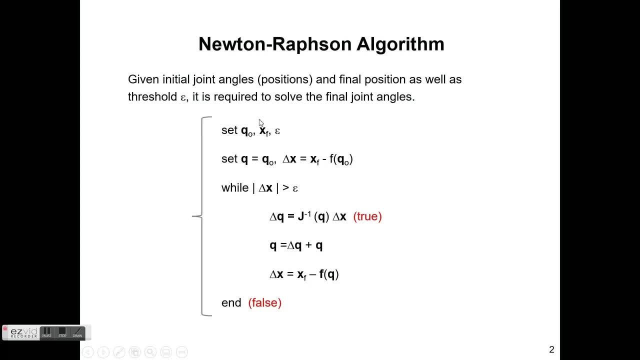 so initially you set the initial angle, final position and threshold, and then, before you do iteration- so this is a numerical iteration method- so you set the q as the initial angle and you can calculate the- uh, the tip difference between final and initial, and then you keep checking. basically, 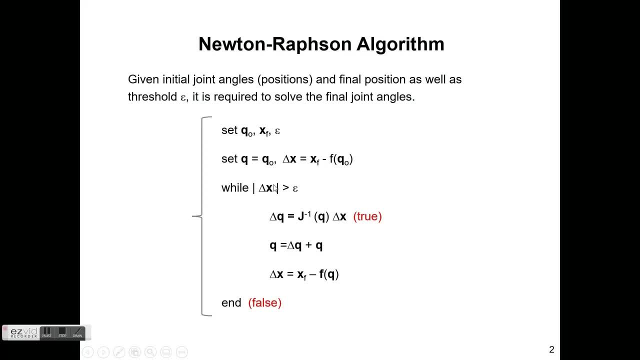 you keep checking the final position and threshold and then you keep checking, basically, you keep checking this, uh, this tip distance, until the q you're trying to solve is close to final q. so if this one is larger than the, uh, the threshold, which is accuracy, uh, the bond that you define, if it's, 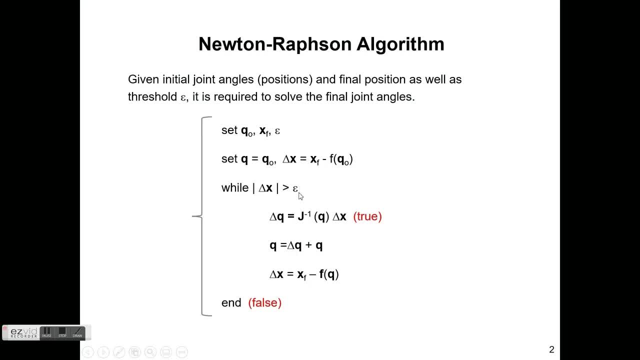 larger, then it goes through the iteration. uh, if it's smaller than this one, which means you find the solution and then you jump out to the slope, so inside the slope, and you're trying to calculate the, the solution, and then you jump out to the slope and you're trying to calculate the. 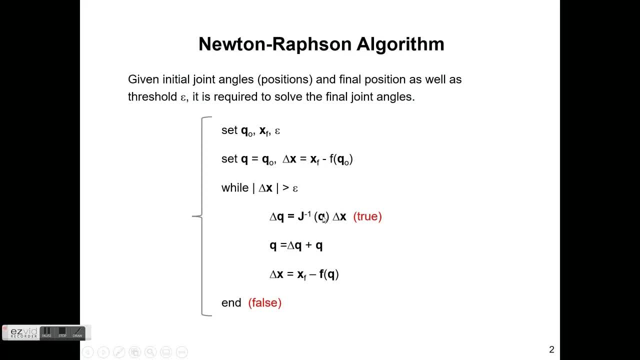 tip difference and uh. this is your copy. i'll show you before. then take your copy English, so you can calculate the uh increment and then you update the, the uh triangle. so this is the, for example. you start from the step one, this will be initial triangle and adding this, this, this increment that you calculate, and it becomes the new. 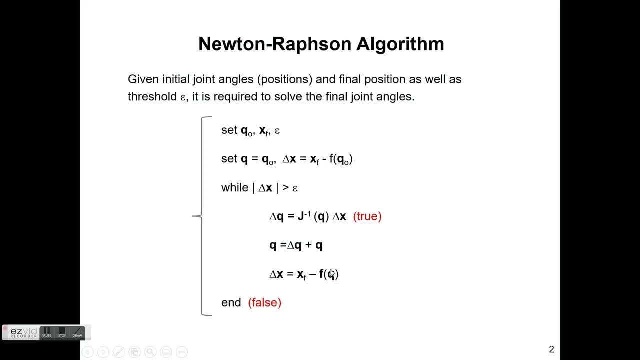 uh triangle and then you put back into the uh kinematic equation and the solve, the position uh corresponding to this angle and then, compared to the desired one, the final, the tip position, and you will calculate the uh, the difference, and then go back if the difference is still larger and then you keep updating otherwise, if this, if this tip error is smaller. 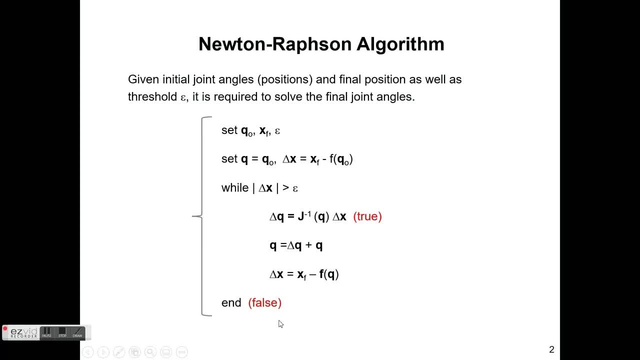 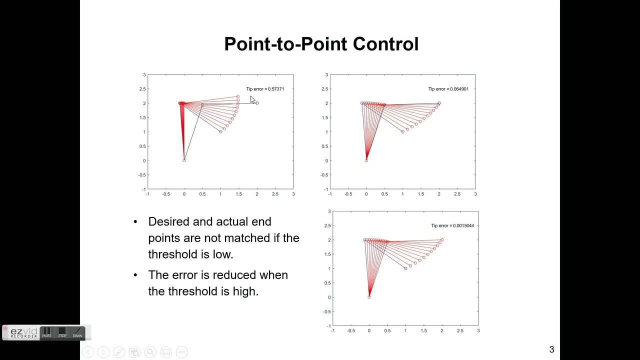 then you define the threshold and then jump out of this loop and here's the example and you see here the. the thresholder, when i define, is small, uh, sorry, it's lower, and your solution is: uh is kind of not accurate, right? and as you increase the uh, the threshold and the iteration gets. 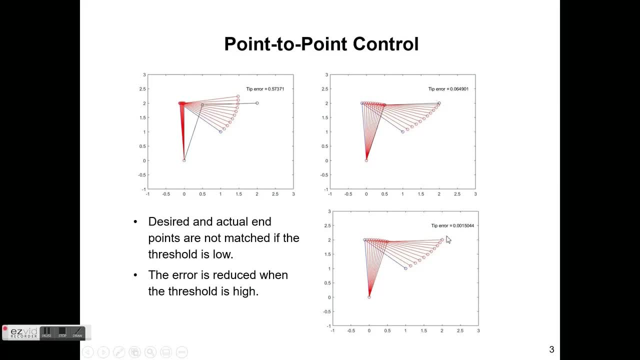 more accurate, like here, and this is even more accurate. so, in other words, if we use the newton rother method, the, as long as you define the threshold, we report the hit points than we do the increment and the anomalia, and that is what this cup about is about. the usualарищ and the around here here and then, as you move up with your left and right, you see that, hoping that if, if there are values right here and then below right in the does match, there is also a right, and here's theремon, but pastry one, which is a vertical way. so you provide sort of you have an LUCA for scholars. 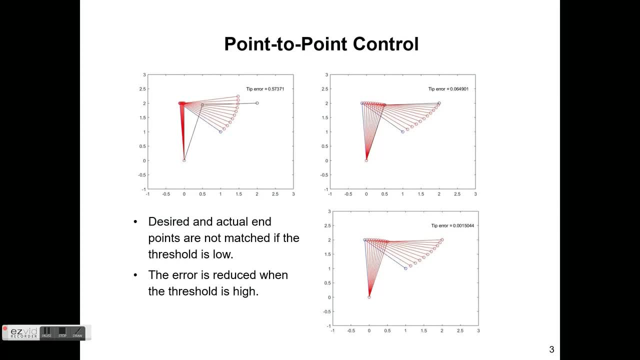 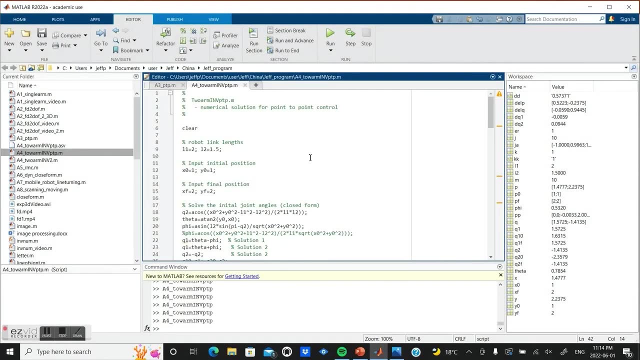 your threshold high enough and you will be able to find the right solution. here is the MATLAB program, so this program is used numerical solution for point-to-point control and, as before, you define the link length: initial position one, one, final position two, two, and because i defined the 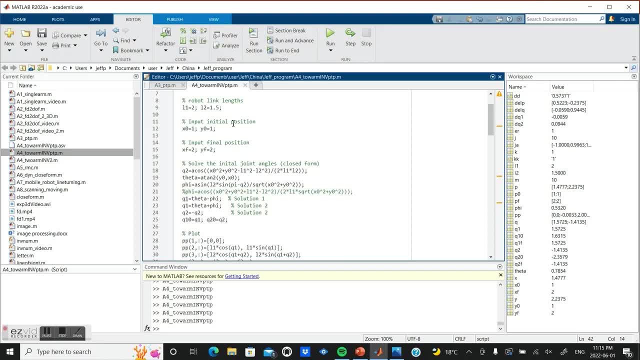 initial, the initial position, instead of initial angle. so here you still can use the, the closed-form solution that i introduced to you in the last video. you can solve this initial angle here and then you plot the- uh, the initial robot configuration, and then use the initial angle as. 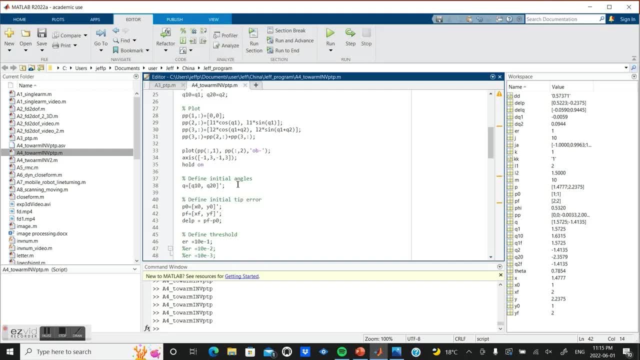 the initial angle for your uh uh atom rafferter iteration and then you define the um. so, initial position, final priority, uh defined input. then you calculate the difference between the two and this is the threshold that you know. it's the error bound you define here is very low. 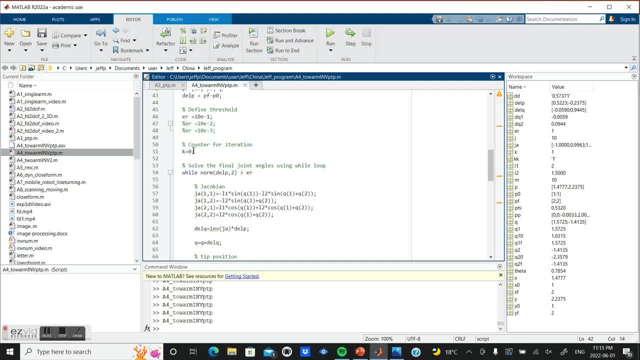 10 to the power minus one, and uh, you can also introduce the counter for how many iterations. and then now you go into this, uh, the loop i just introduced you in the power point. so first you calculate the jacobian and then then calculate the, uh, the joint angle increment, and it updated the joint angle, and then you put into forward. 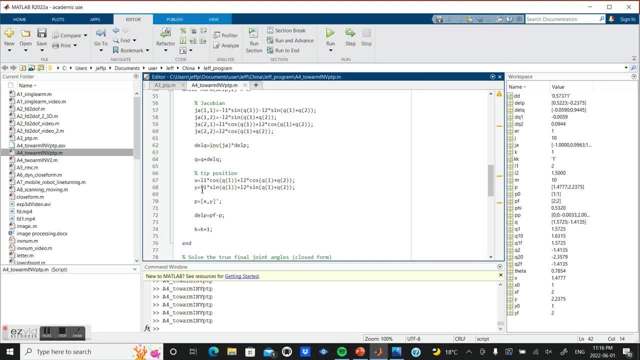 kinematics to calculate the tip position x or y, and then you compare where is the final? there's a p final against the current one that you calculate, and then you update your counter and if then this program will go back to here, see if this one is larger than the arrow body defined. if it's a. 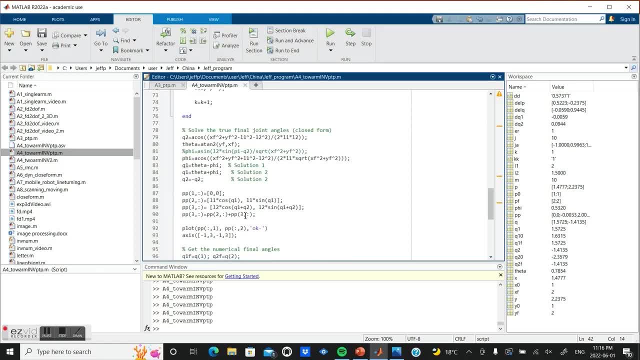 p, then you can go slow this uh the slope again. and here i use the closed form solution here again to calculate the uh the true, uh final angle, just to check with the uh the accuracy, okay, and uh, that's what i showed you last time. so this is the sort of closed form solution and then you calculate. 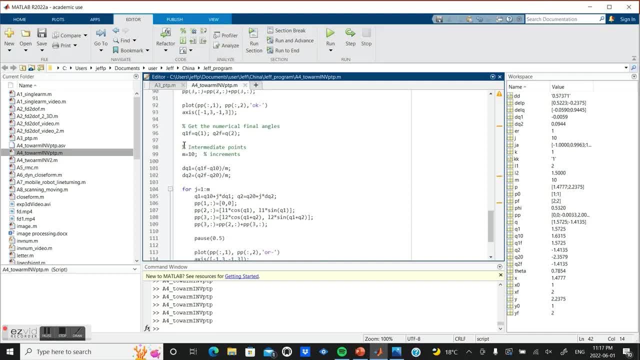 and then your plot, um, and then here, uh, you're getting the numerical final angle. you want to find the angle, and then then you calculate the difference between the final and the initial, and then for joint one, joint two. so basically you can calculate the intermediate points and then use the four loop again like, uh, the one show you in for the closed form solution. 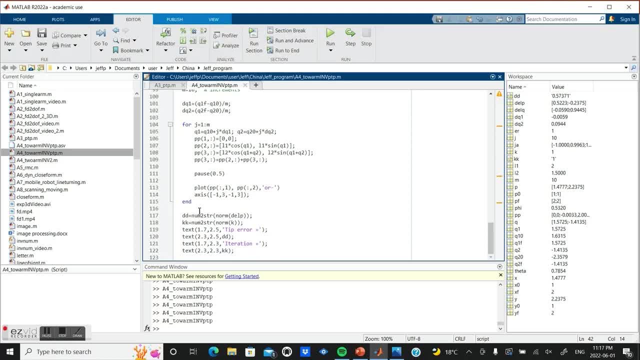 and you can go through the intermediate points and here you just uh, i just show, uh on the plot, um, the the arrow, final error, how many caps? so i'm going to show you here. the first case would be: the arrow is a relative larger here. this one, this one here, so i can show. 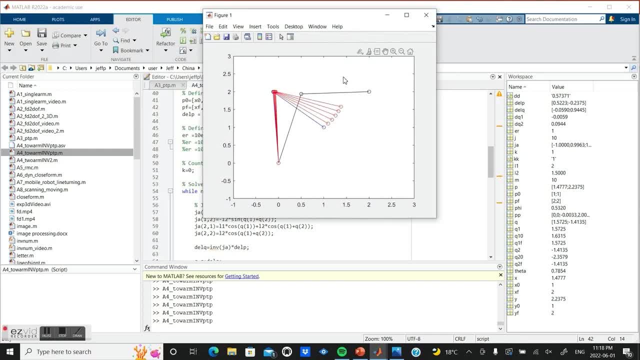 you here, because the arrow balance is a relative low. so that's why your final iteration, your arrow, this is the initial position one, one is the final position, two, two. but so iteration, your final position is here. so if your error bond is lower, and then your solution will not be accurate. so 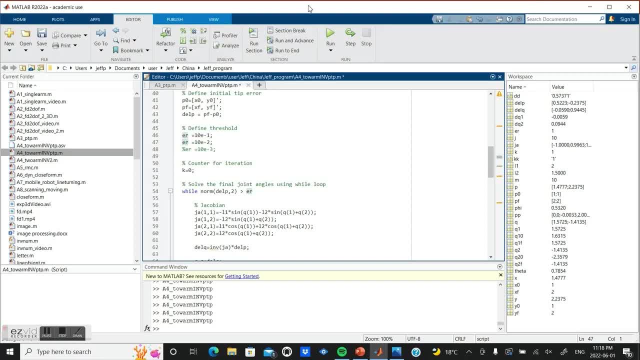 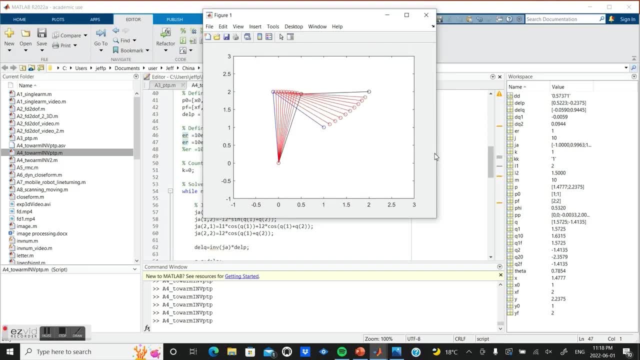 let's say, we increase the error bond again. so now, obviously, it's getting closer to the true value. here again, this is one, one, this is two, two. right, let's turn to here, this one. here the arrow is getting smaller. and the first one i show you. 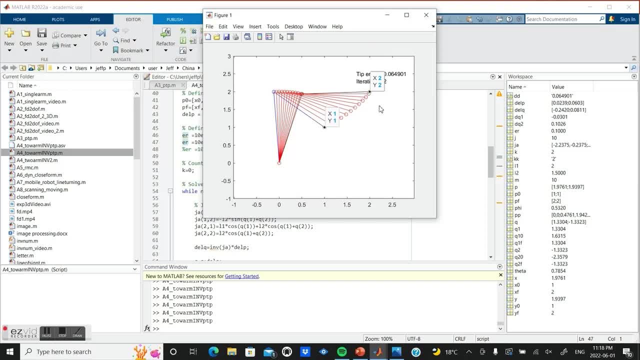 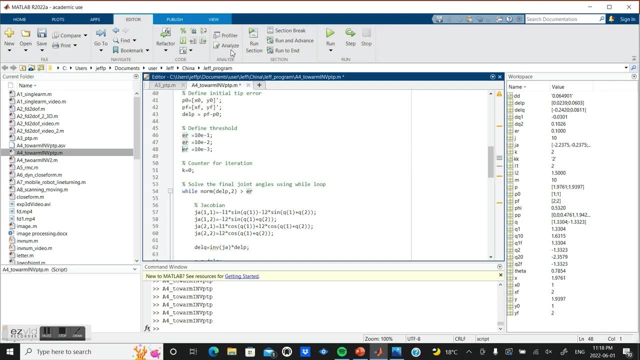 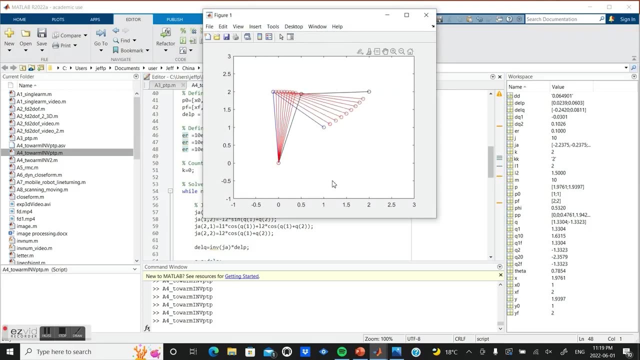 is just one iteration, this is for two iterations and that would be two, two, right, so then keep increasing the little one. okay, this is more effort. and then you run again. so this is very accurate. see, the arrow is is a, really accurate. and then this is those three iterations and you can see this is the initial. 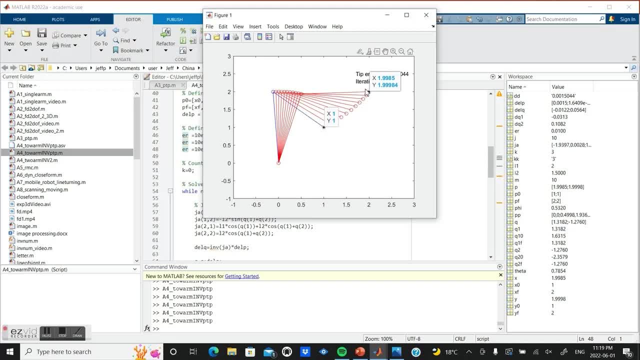 position and this is very close. right, the final position is very close. okay, i hope you learned something from this video. 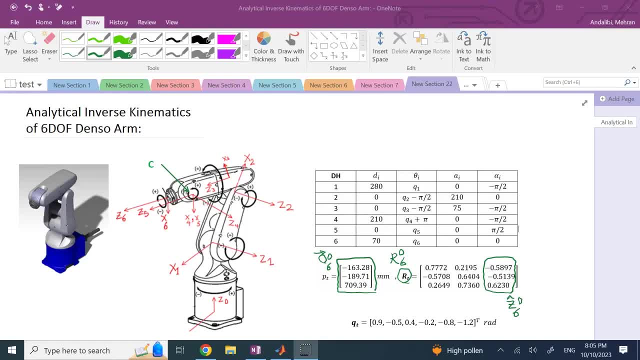 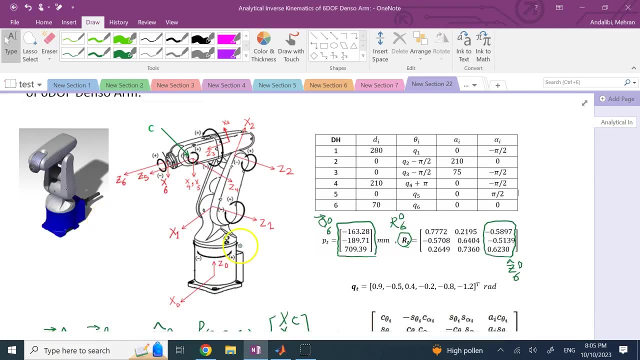 Hello everyone. In this video I want to show you analytical inverse kinematics for the 60 OF Denso robot, This robot that you can see here. It has six degrees of freedom. as you can see on the right side, All of them are rotary right, So you.